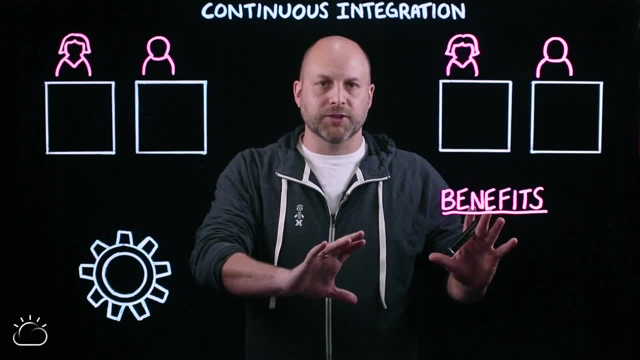 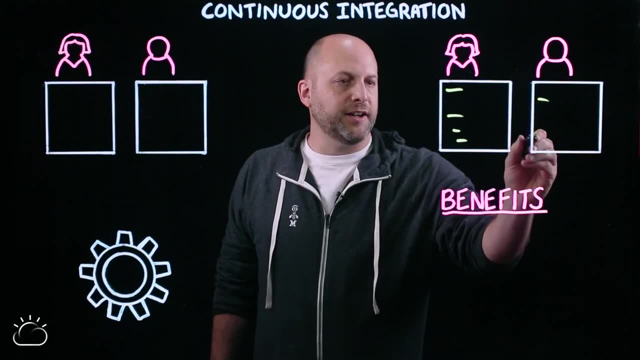 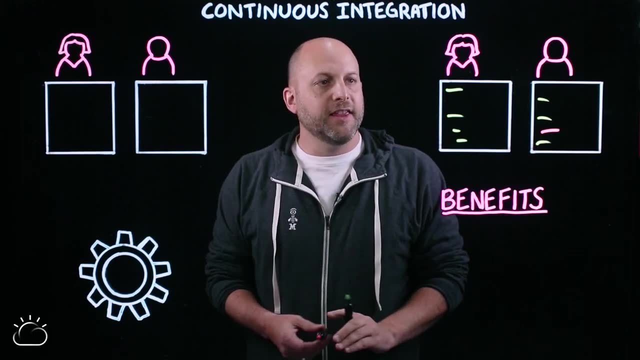 features and they're going to keep separate on their own features for a long time, right? So you know they're writing some bits of new code here. You know, maybe they're they're deleting a line of code here or there. what have you? And their plan is that they're. 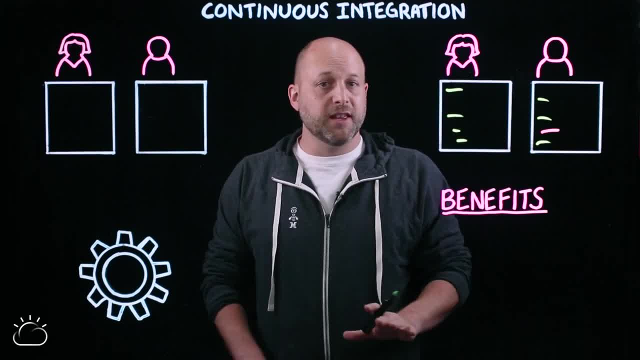 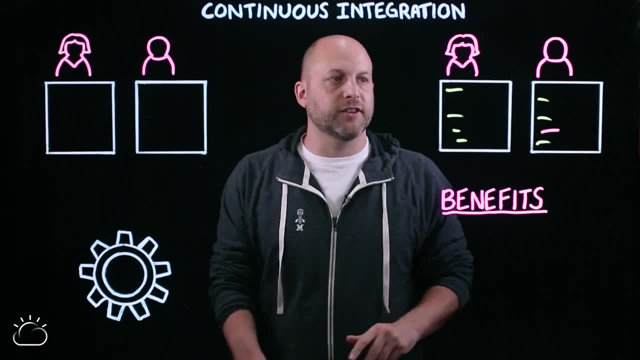 going to get their features to work against the code base and then, a couple of weeks or months later, they're going to integrate their work together. They're going to merge their work together. They're going to say: my code, your code's got to come together, it's all got to work. 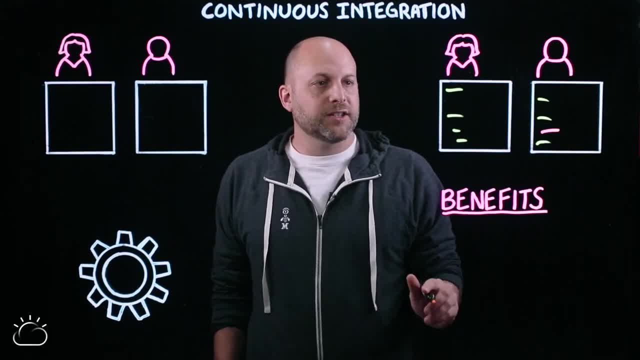 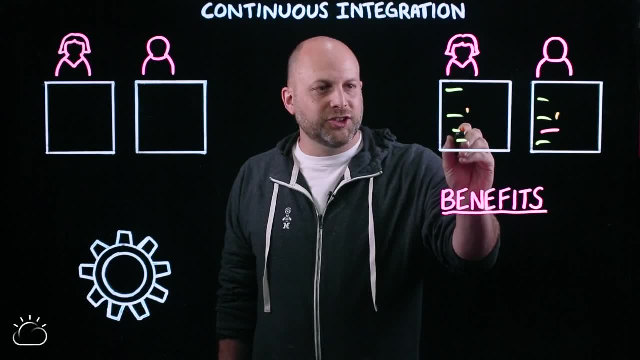 Now in this world, you could have a situation where Alice and Bob- well, they changed the same line of code, but they're going to get their features to work against the code base. They're going to get their features to work against the code here, right, And maybe Alice changed this code. 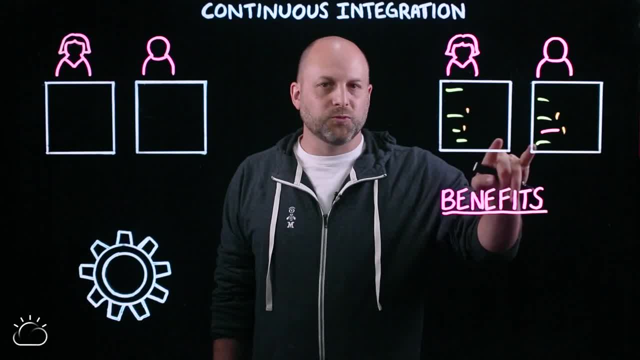 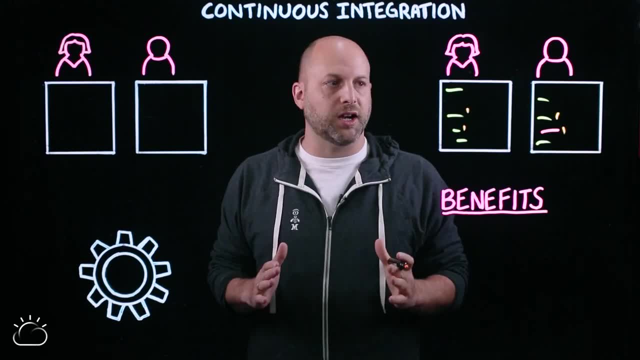 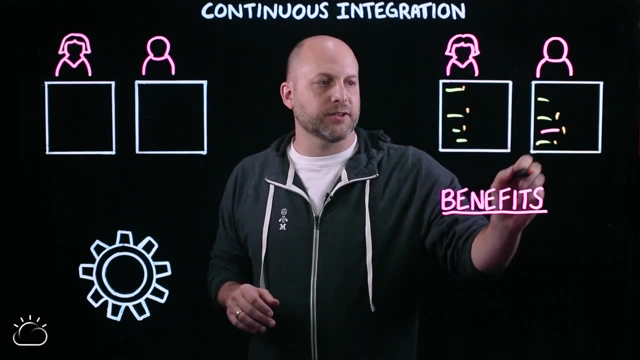 but then Bob deleted it, And so this gets really awkward really fast. when you just try to algorithmically combine it right, You get what's known as a merge conflict. This gets worse because it might be that some code up here interferes with some code down here. 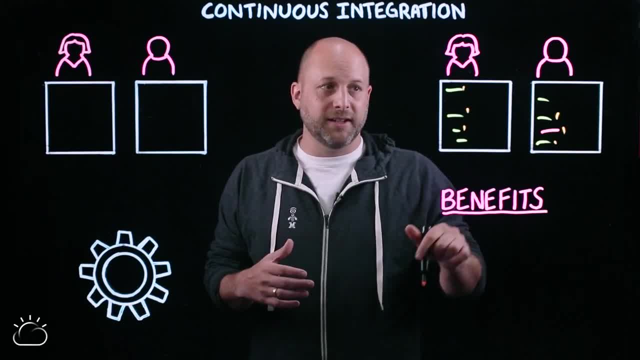 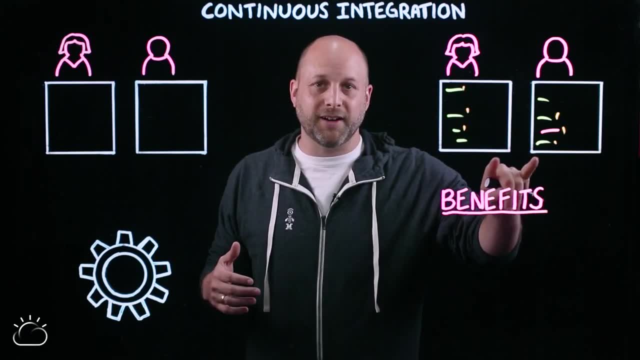 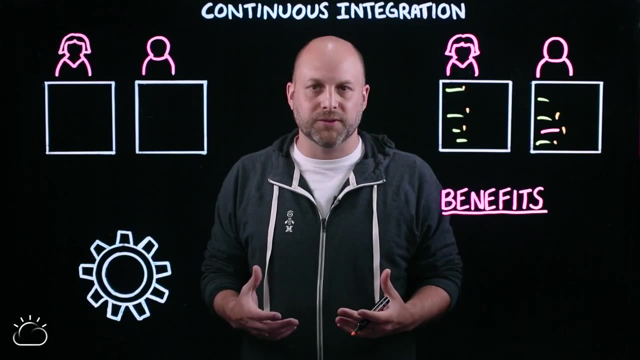 They just don't work together and you've got bugs, And this will happen here within just one file, but in the real world it's not just two developers working on the same file. There's thousands of files or millions in an application. There's tens of developers. 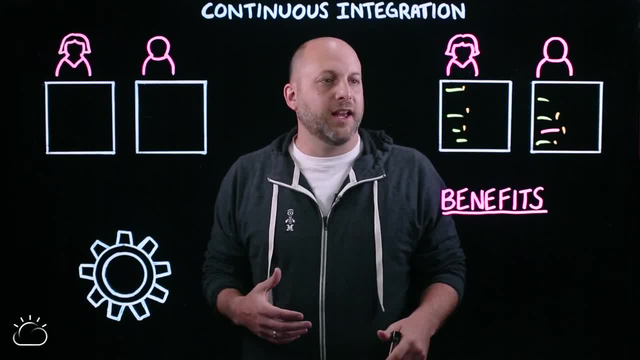 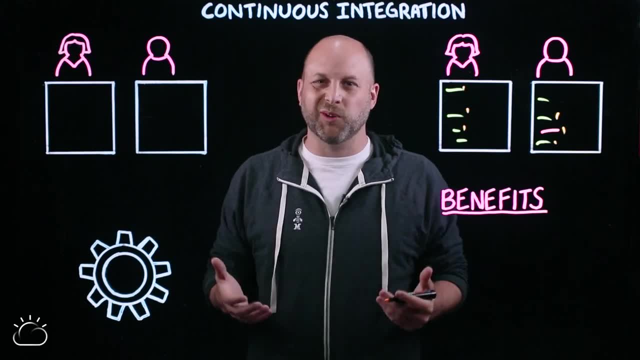 involved and they're doing this over weeks and weeks And so, reconciling all of these problems, big mess called merge hell. And so it's like, well, what do we do to avoid merge hell? This is how we got here. Well, we start and we'll have Alice write the code here And you can see Alice. we're going to do the nh2 hash tag, the hash tag that we found in this code, and here's an example of the hash tag configuration we found, And so we're going to call this hash tag configuration and we're going. 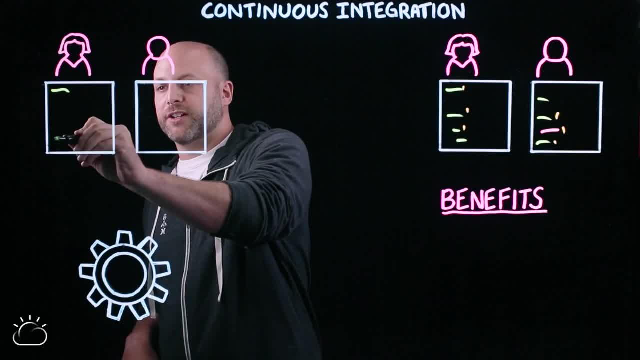 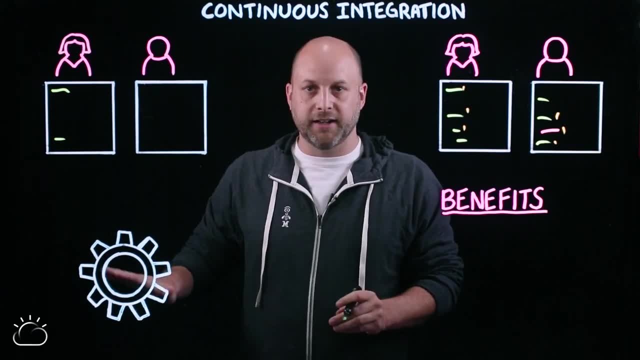 to call it the hash tag configuration right now. And we're going to call this hash tag configuration. And we're going to call this hash tag configuration writing some code again. right, Alice writes her code. cool, as soon as she has something that works, even a little bit, her feature is not done, but she's got. 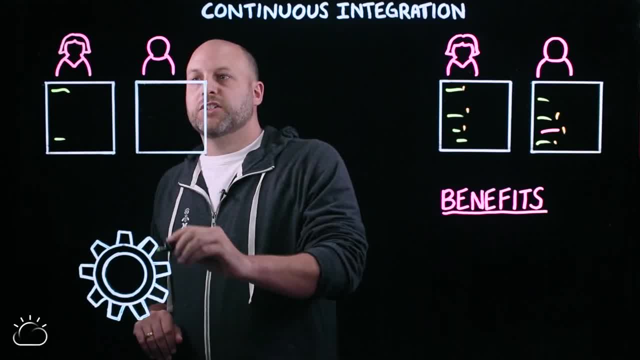 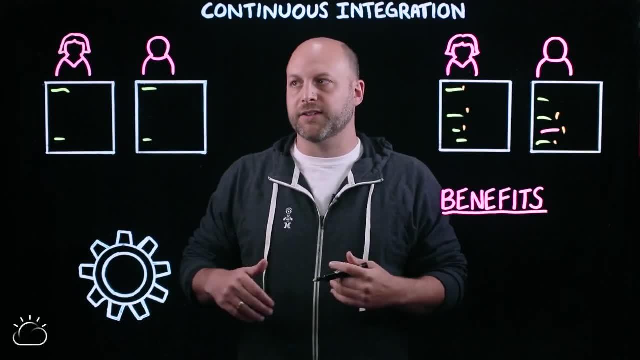 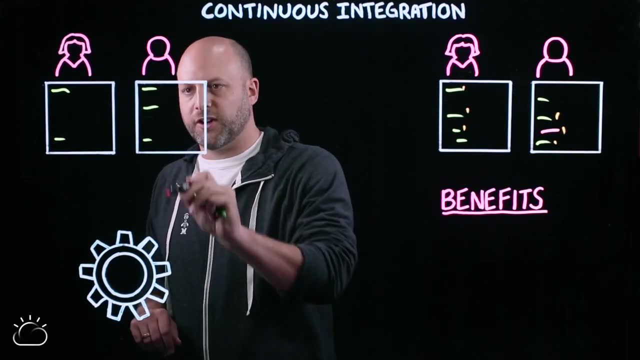 code that works. it doesn't break things. she submits that in the source control. Bob pulls down the same code before he starts working. right, he always is working off. the latest Alice is always submitting hers in. Bob makes his change. all right, maybe he deletes a line of code. great Alice comes back. she's. 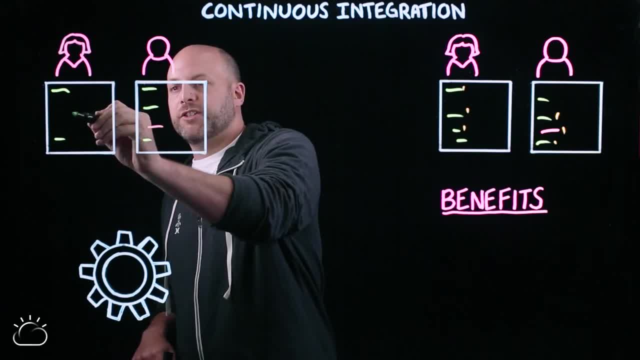 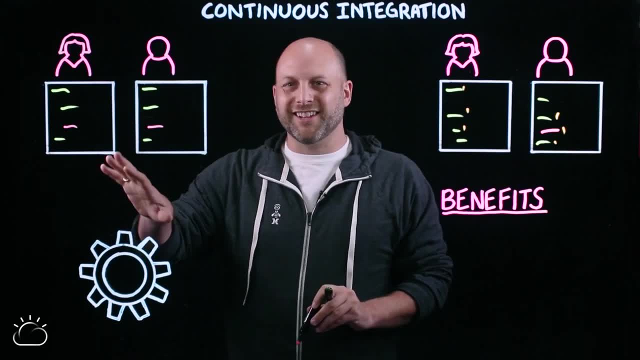 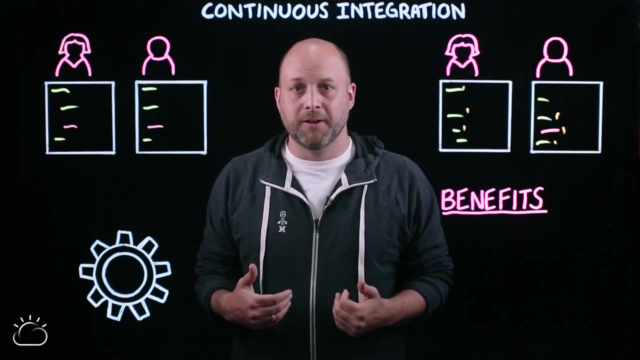 working on another part of her feature. she's working on another feature. she grabs Bob's code- cool, and now they're working on these things together. in the likelihood that they're both working on the same thing at the same time and that they conflict, it's pretty small and if they do hit that, it's all on code. 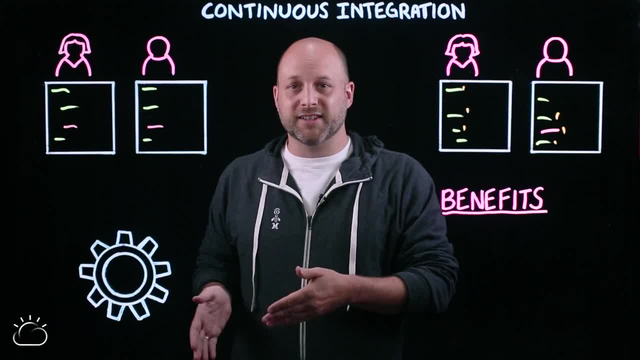 they've worked on in the last day. you're going to have to make sure that they're working on the same thing at the same time and if they do hit that, it's all on code. they've worked on in the last day. but right, they can sit together and they can reconcile this thing. it's no big deal. 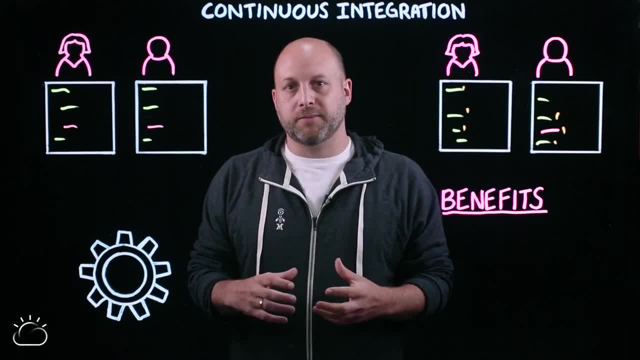 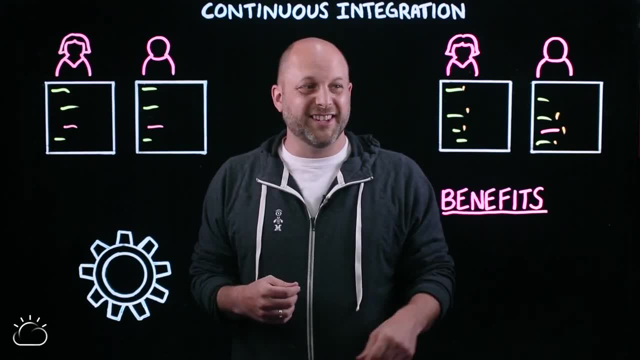 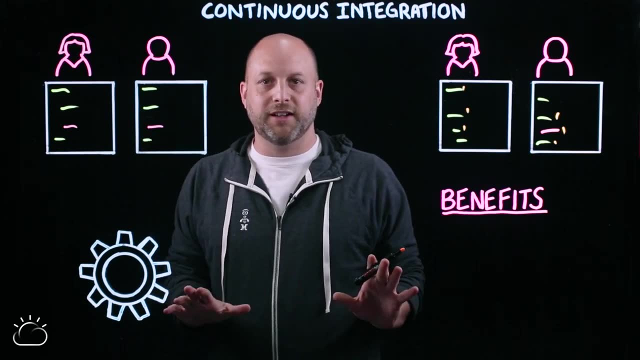 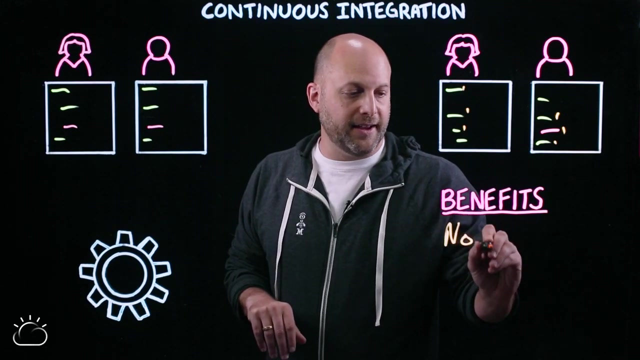 and so the core principle that we're seeing here- one of my favorite things in software development, because it's so counterintuitive- is that if it hurts, do it often and it won't hurt so much, and that helps us get rid of the big, big bogey here, right, which is, you know we're going to not have merge hell. 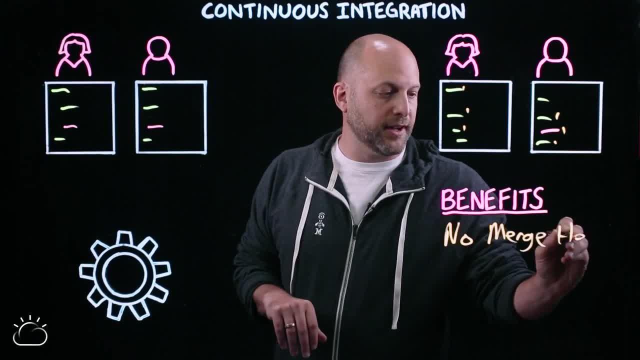 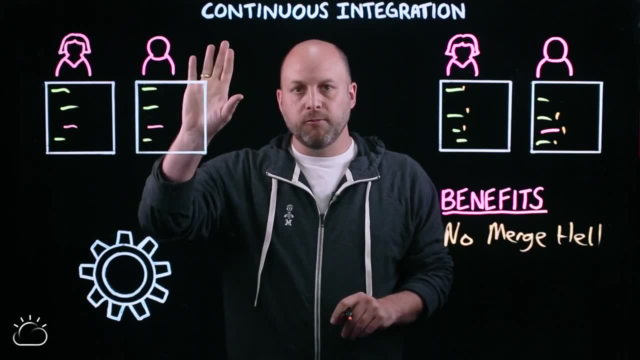 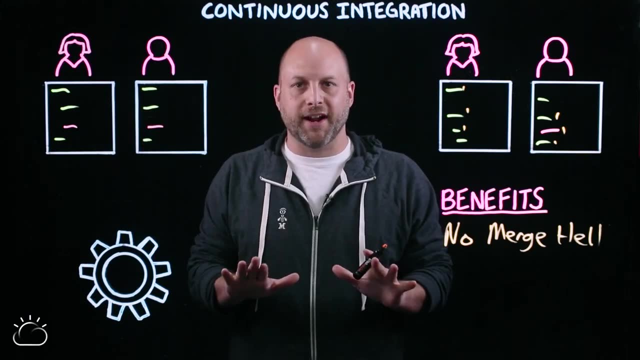 we don't like merge. hell, get rid of that. okay. so that's, that's fixed number one. now this does create a new problem, right that have a whole bunch of people constantly checking in code into the code base. things are going to break, right. it's not going to compile. there's going to be bugs that weren't there. 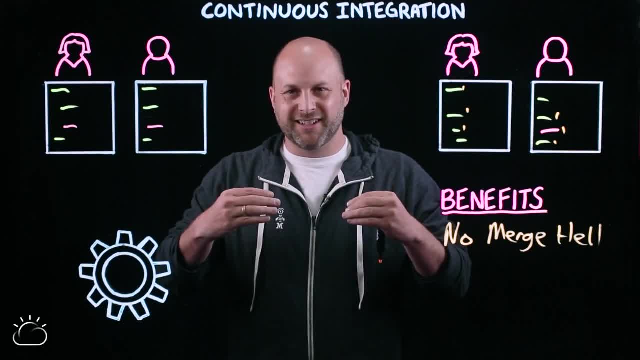 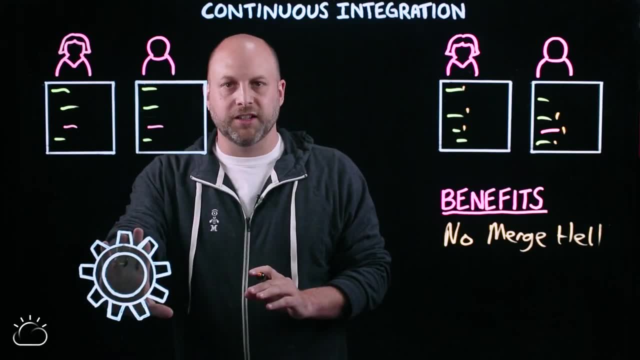 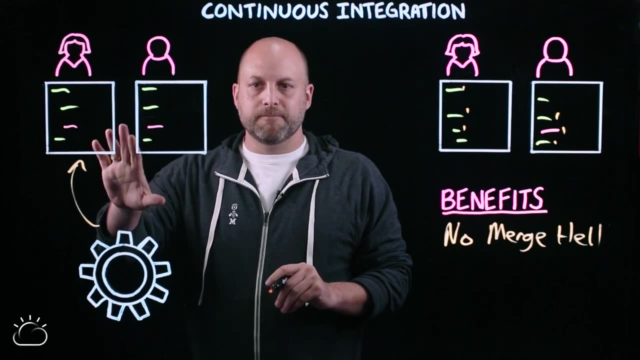 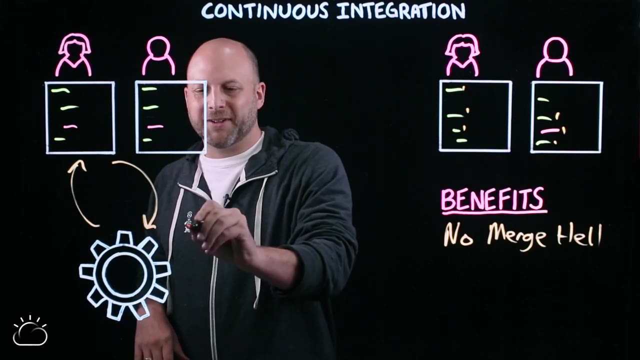 yesterday and you have. this kind of continuous integration led to continuously broken problem, and that that's sad. so what do we do? well, we put some automation in right and it's always watching the code, keeping an eye on it, and whenever a change happens, says: okay, let me grab that code, i'm going to build it and then i'm going to.